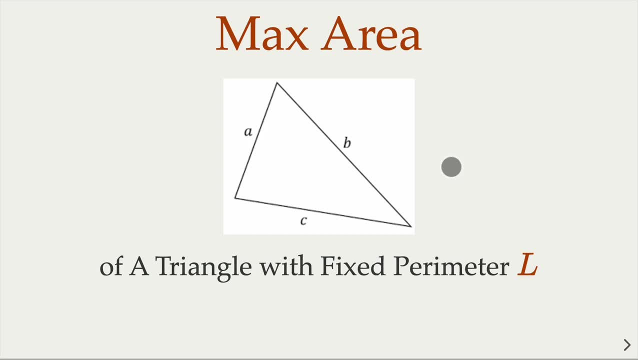 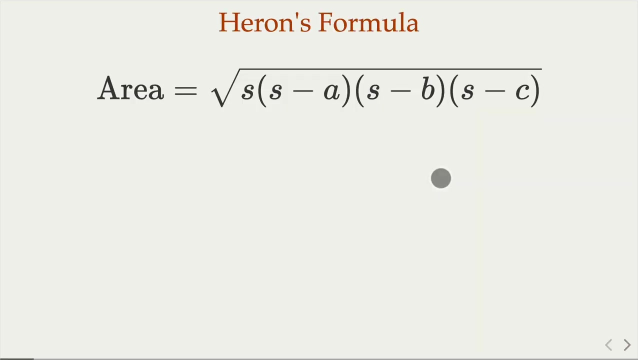 We look at this classic problem of finding the max area of a triangle if the parameter is a constant L, That is, in this diagram the A plus B plus C equal L, and we try to find the max of the area. We know Herron's formula relates the area to the size of the triangle where S is half of the. 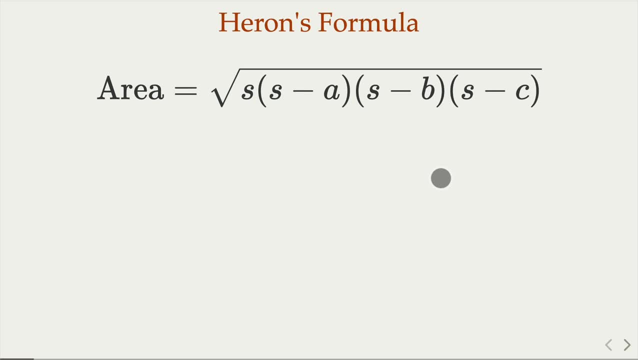 parameter, that is in our case S, would be a constant. that is half of L, that is half of A plus B plus C. We need to find such that this area is maximized. We are going to use inequality, that is for n real numbers here positive. 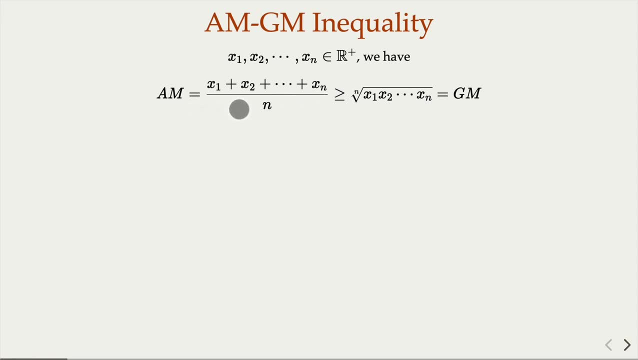 the arithmetic mean, that is the average, is going to be greater or equal to the geometric mean, that is the average. And then we are going to use the nth root of the product. here We are going to use n equals 3.. 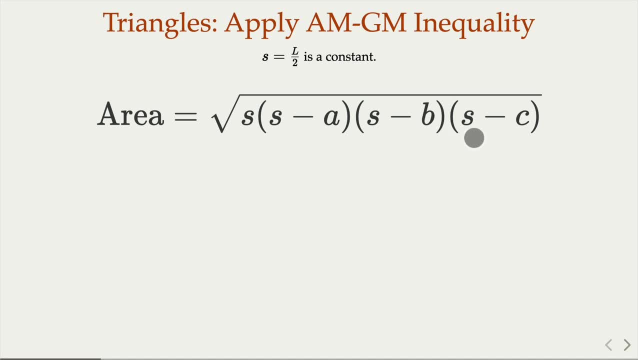 This is constant, so we care about these three terms. here Apply the AM GM inequality. First, we note that this is cubic root and also the right-hand side can be simplified. That is S minus A plus B plus C over 3.. Of course that is, S is half of L minus L over 3,. 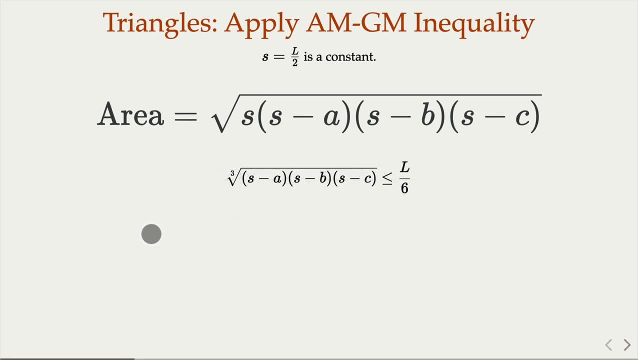 that is L over 6. What we have is this: Now you want to make cube of both sides. Here in the formula we have S, so we would like to multiply S on both sides. S is half of L, so plug in to the right-hand side. 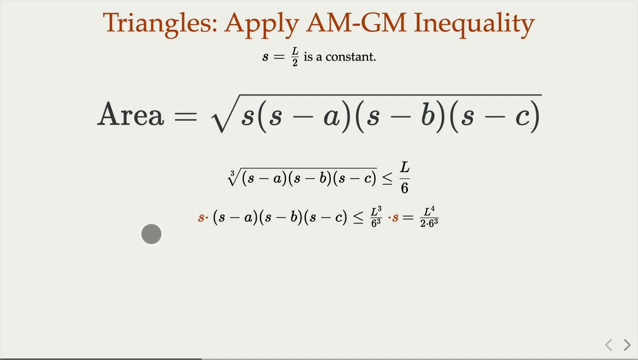 you're going to get this Now. the area the quantity is going to be square root of it is going to bounded by this upper bound. Now, the equality holds when the three quantities equal to each other- A, B, C- are equal. That is, the maximum is achieved. We have the maximum when 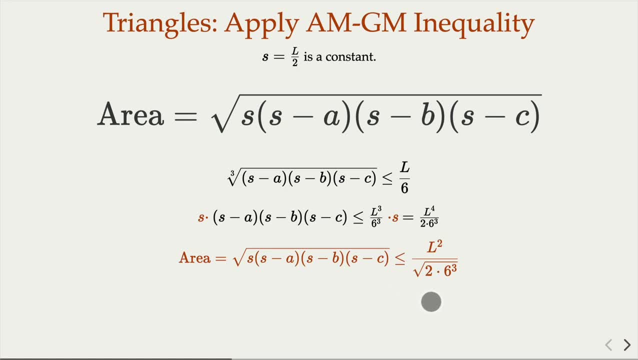 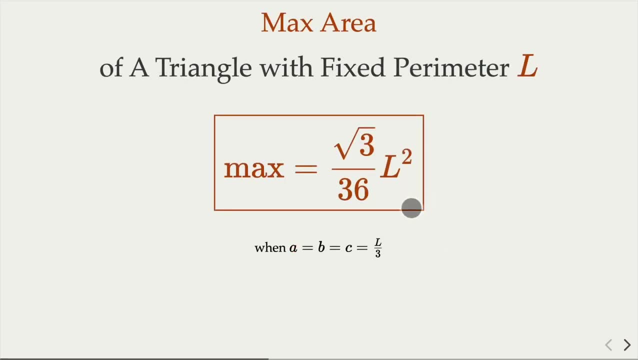 the triangle is regular triangle. You can simplify this quantity here. It's going to be this, All right, so our final answer. So this is the max value with fixed parameter L. This is achieved when the triangle is regular. So today we review this well-known result.